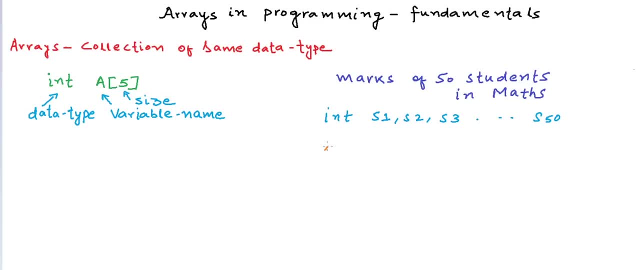 Let's say we want to calculate the average marks of all the students. So to calculate that, we will have something like a total of all the marks, So we'll have a variable total, and then this total will be equal to S1 plus S2 plus S3 and all the way. 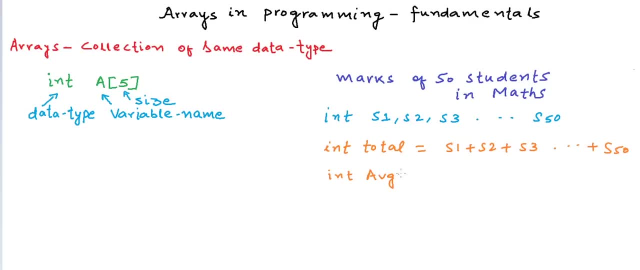 till S50 and average would be total divided by 50. But what if we had 500 students or even more? It would be very unmeasured. It would be unmanageable to declare 500 different variables and use them in our statements. So in these cases we declare: 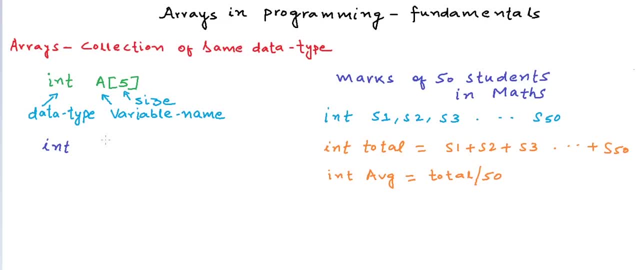 an array. So let's say we declare an array S with the size 50 and this array is an array of integers. Now, in this case also, I have 50 different variables and I access them as S0, S1, S2 and so on. We start at. 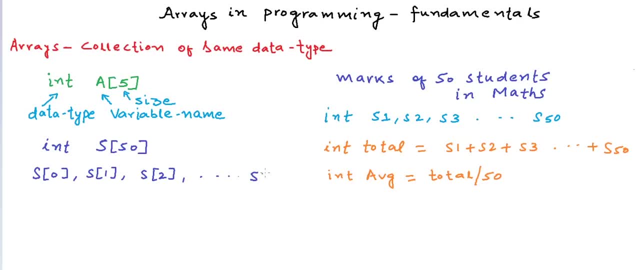 index 0 and we go all the way till index 4.. And our program will be something like: we again have a variable total, and this time we run a loop from 0 to 49 and we use the variable i as index and keep on adding. 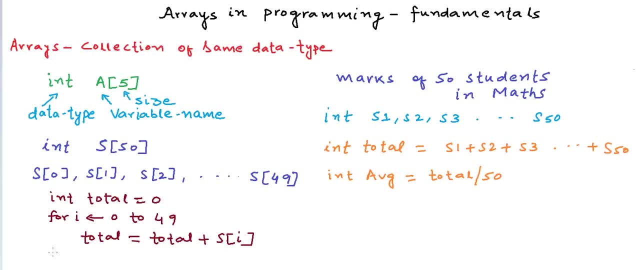 Si to total. and finally we return or calculate average as before, which is total upon 50.. This was an array of integers. We can also have an array of float or an array of character or an array of a user-defined class or structure, And this was 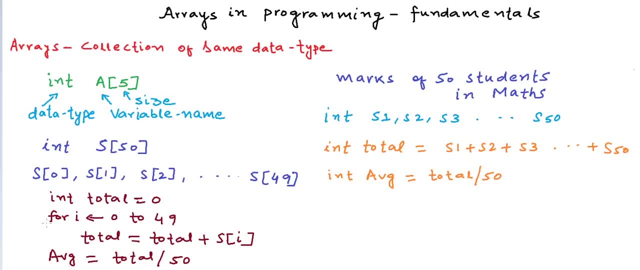 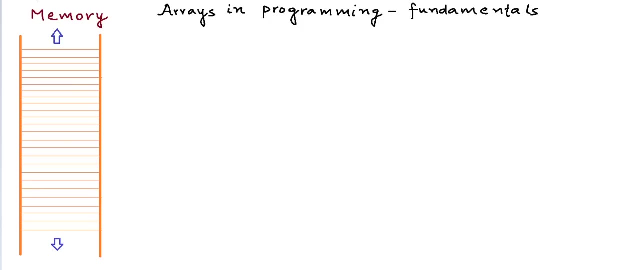 a simple one-dimensional array. We can also have arrays of two-dimension or three-dimension. Let us now see how arrays are stored in computer's memory. Okay, so let's say this figure in the left here is computer's memory, which is divided into these segments or partition. 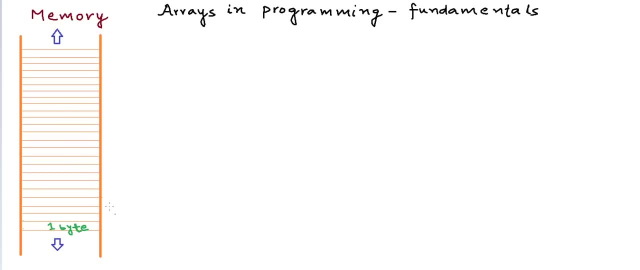 and each segment is one byte of memory. In fact, we are only showing a part of the memory in the form of these segments or partitions, and that's why it is extending towards the bottom and the top, because, in reality, the memory will have many more bytes, In fact. 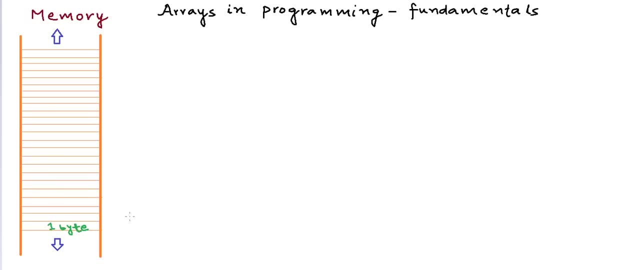 computer's memory is a very large array of bytes. Now in computer's architecture each byte of the memory has an address. Let us assume that here, the bottom most byte, which will be somewhere deep down here, has address 0, and as we go on towards the top we keep on increasing the address, like 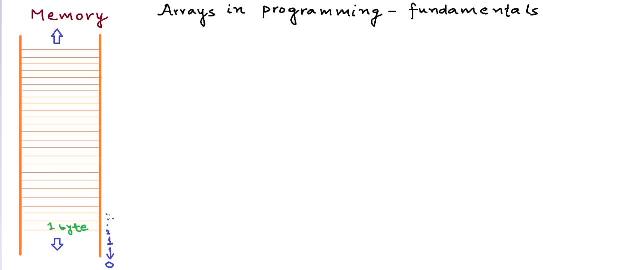 1, 2 and so on. So let's say, for example, if this particular byte has an address 100, then this particular byte will have an address 101, and we will go on like 102,, 103 and so on. And as we know, in C or C++ we can also have 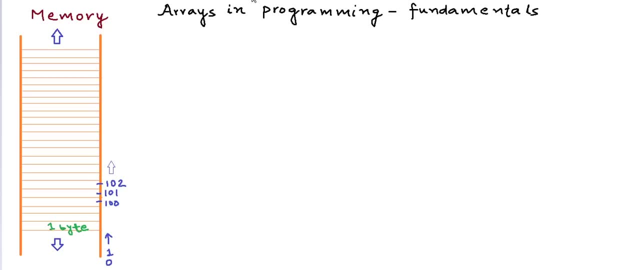 pointer variables that can store the address of another variable. Now when we define an array, something like an integer array, let's say, for example, of size 4, then if an integer typically takes 4 bytes of memory, then an array of 4 integers will take. 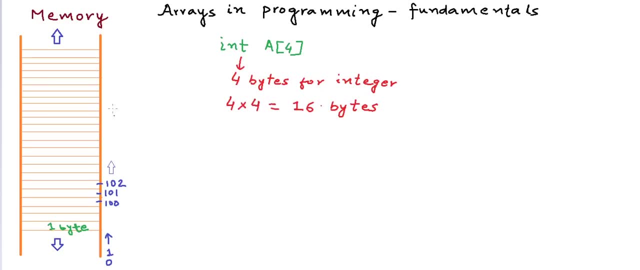 16 bytes of memory. When the program executes, the computer allocates 16 contiguous bytes in the memory for this array A. So the computer kind of allocates 4 contiguous blocks of 4 byte each. The first block, or the first 4 bytes, will correspond to 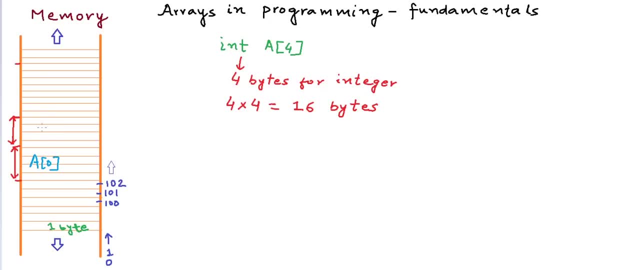 A0 and the next 4 bytes, or the next block, will correspond to A1, and similarly we will have A2 and A3 as well. Now, access to an element in the array or its modification. all of it, all of these operations take constant amount of time. 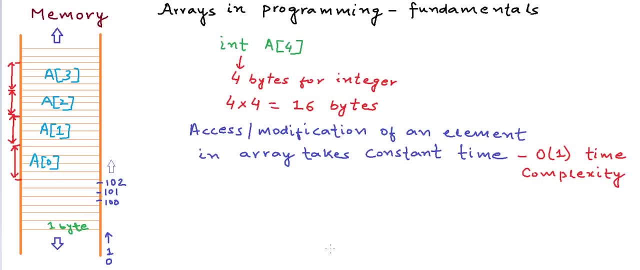 and it is not a function of the size of the array. or in other words, we can say that the time complexity for accessing or modifying an element in the array is O. Now how does this really happen? let's try to understand. when we declare an array like 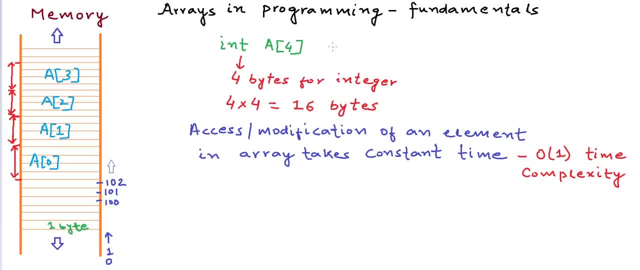 say, for example, here we have declared an integer array of size 4, then this variable A is nothing but pointer to the first element in the array. and we can also say that this variable A is a pointer that points to the base address of the array and this: 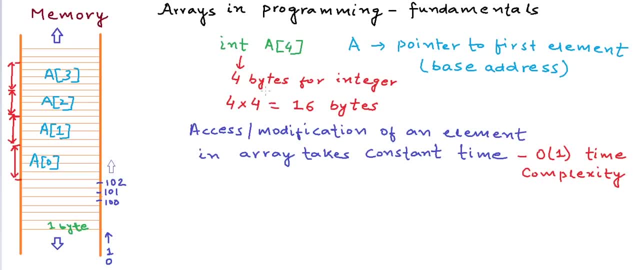 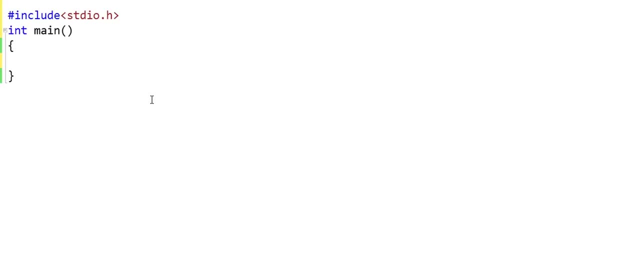 is better explained in a real program. so let us go to a compiler and write some code. So I will write a simple C program here. what I will do is I will declare an array A of size 4 an integer array. So I will declare an array A of size 4 an integer array. 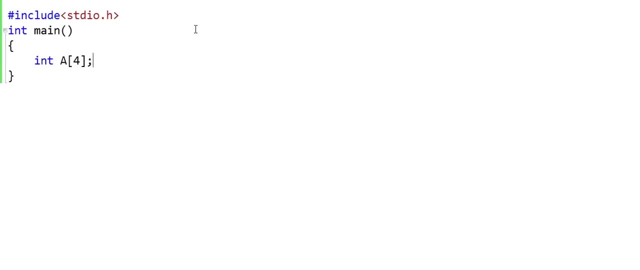 So I will declare an array A of size 4 an integer array array And, as I told you earlier, a is nothing but a pointer to the first element in the array. So if we try to print a and I have written a simple printf statement which is: 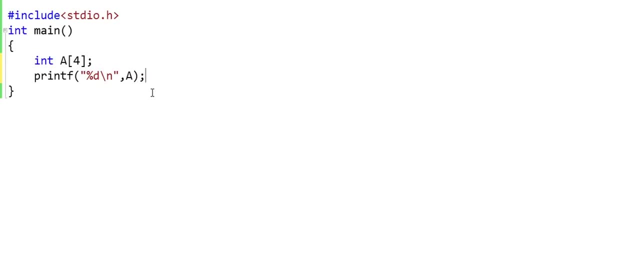 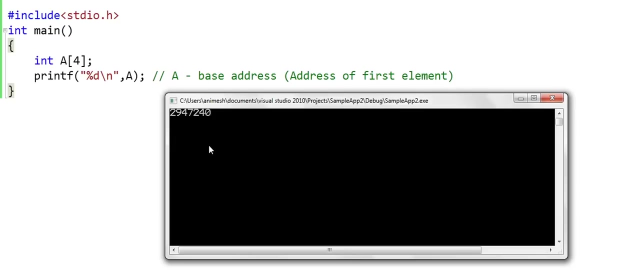 the statement to print a variable on the console, then this should give me the base address, or the address of the first element in the array. Let's now run this program And we get an output which is equal to 2947240.. And this should be the address of the first. 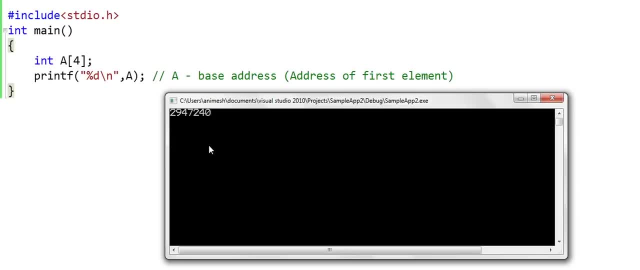 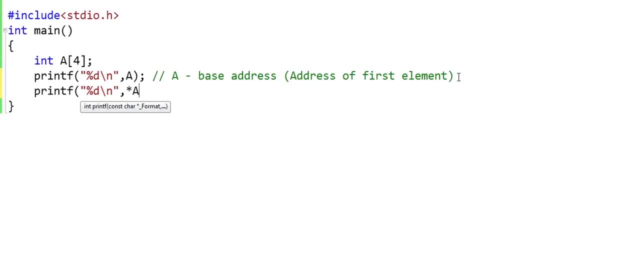 element. But how do we know that this is the address of the first element? Well, we can print the value at this particular address And, as we know, to print the value at an address a pointer variable points to, we need to put a star in front of the pointer variable in. 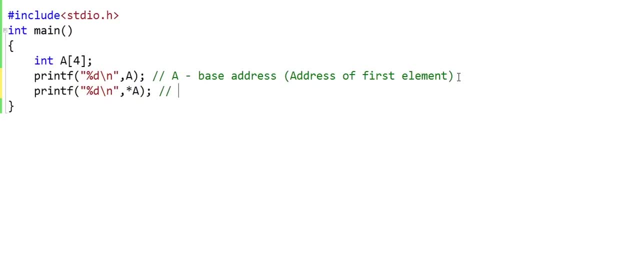 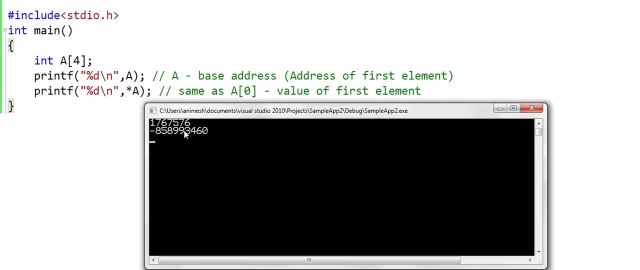 C or C++. So star a should give us the value at the base address, or the value of the first element in the array. So star a is same as a zero. And let us now see what we get. Okay, so we got an address in the first line And this: 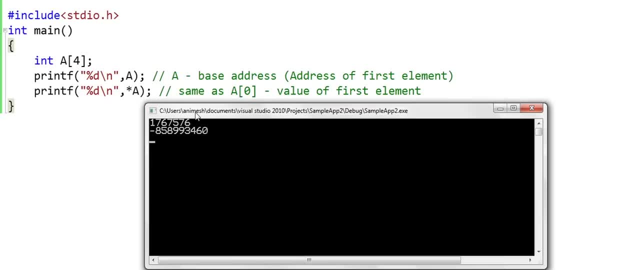 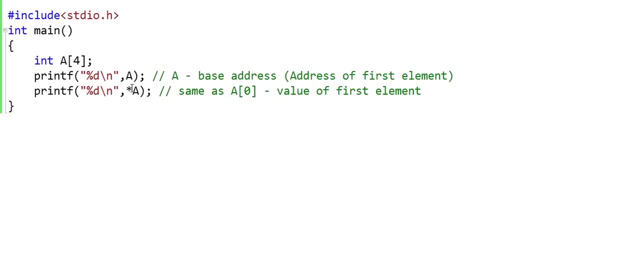 address is different from the previous address because every time the program runs a fresh, the memory allocation will be different And the value that we are getting is some garbage value. This is happening because we have not yet initialized or filled any data in the array, So what I'll do here is I'll fill some data. let's say a zero is one. 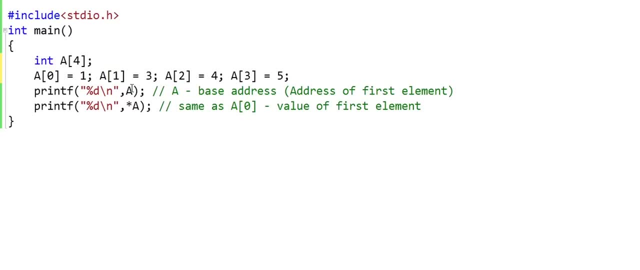 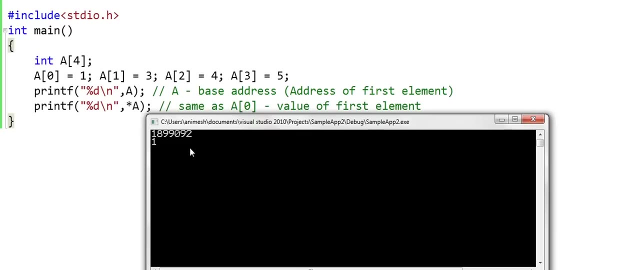 a one is three, a two is four and a three is five. And now if we, if we run this again, the first line once again gives us the address of the first element And the second line gives us the value of the first element. And that's correct. Now I'll do something else. 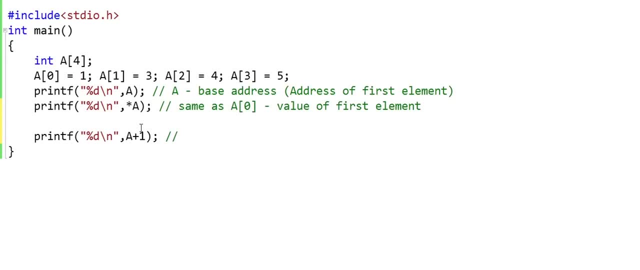 here I'll print a plus one, And if we know the basics of pointer arithmetics then we'll do this. Then, because a is a pointer to an integer, then a plus one should increment the address by four bytes, which is the size of the integer, and take us to the next integer. 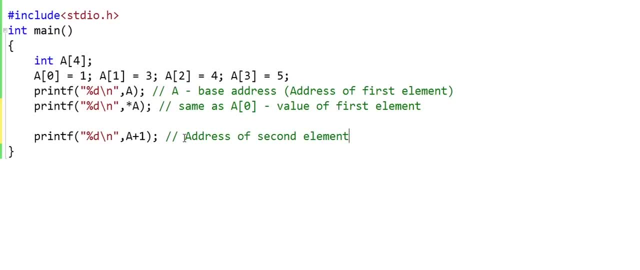 So a plus one should give us address of the second element in the array, And whether this address is correct or not is something that we can verify by looking at, looking at the value at this particular address, And if I'm all right, then this should: 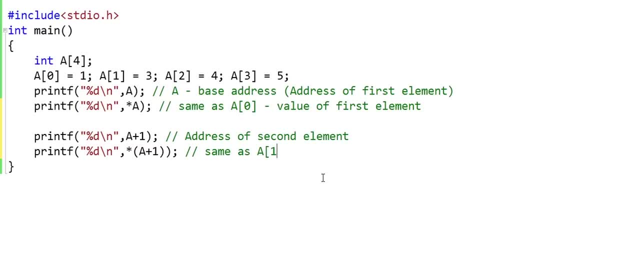 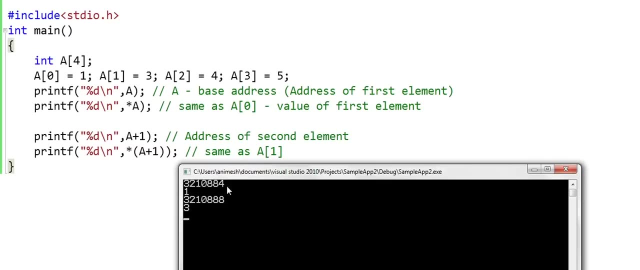 be star of a plus one should be a one or the second element in the array. Let us now run this Okay. so first line is the address of the first element And, as we can see, the second address, which is the address of the second element, is four more than the address. 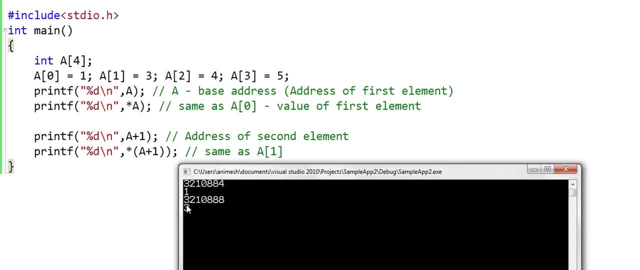 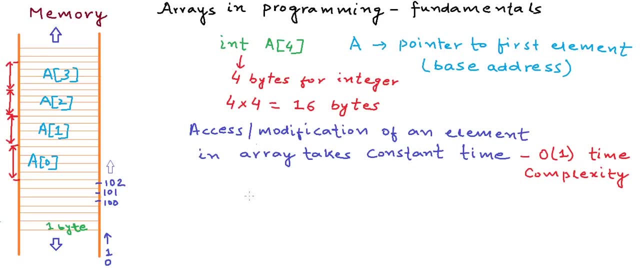 of the first element. And we have got the values right. a zero is one and a one is three. So now it should be evident why accessing or modifying an element in array takes constant time. So if we want to access an element in the array, the computer first calculates the address. 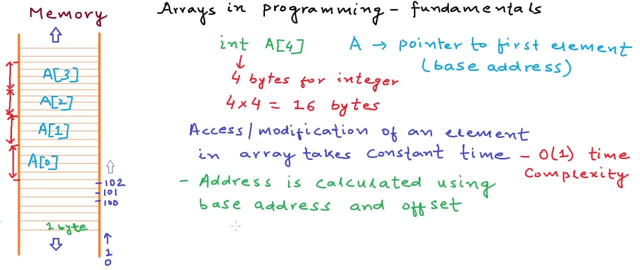 of this particular element using base address and offset. So, for example, if we want to access the fourth element in the array, which is a three, then the address is calculated from the base address a, by adding the offset three and the value at this particular location. 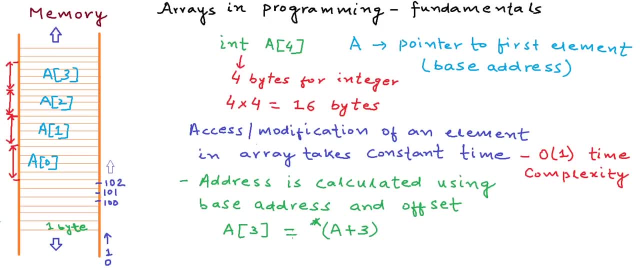 will give us a three. all these pointer arithmetics that we're doing here are possible only in C and C++, And if you are using a language like Java, you do not have explicit pointer variables. But still, the internal working of how things happen in memory will be pretty similar. So 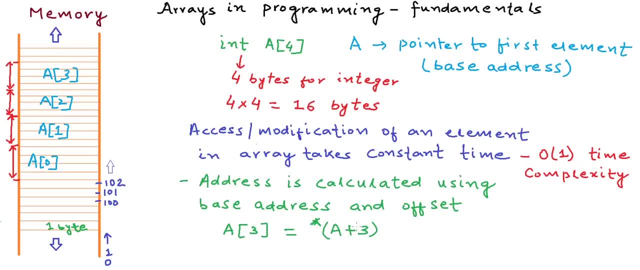 this was some of the basics about arrays and how they are stored in memory and how they are interpreted in a computer's program. In the coming lessons we will talk more about arrays and solve a couple of problems. So thanks for watching.